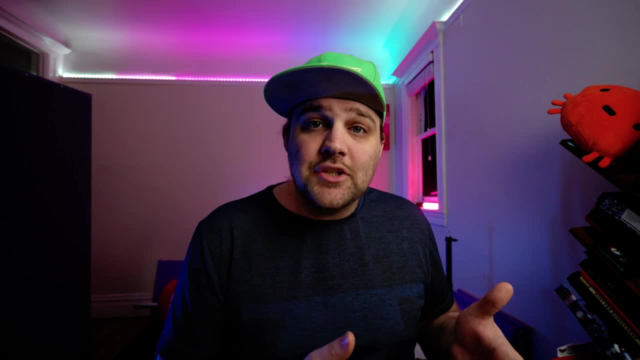 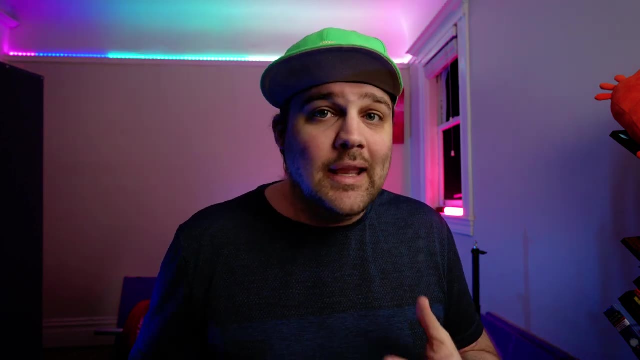 another video. So suffice it to say that this deep integration means that you can access the ecosystem of sort of middlewares and other routing functionality, such as timeouts, rate limiting, load balancing and anything else. you want to write Many of this middleware or additional. 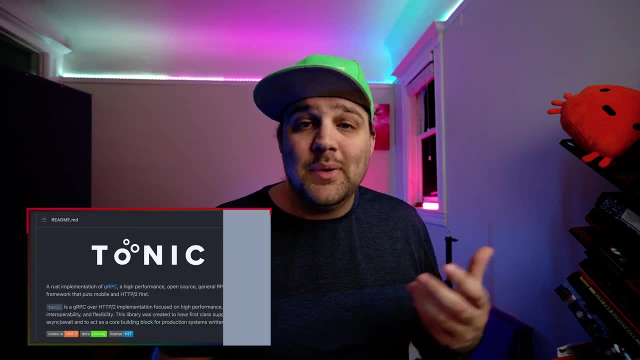 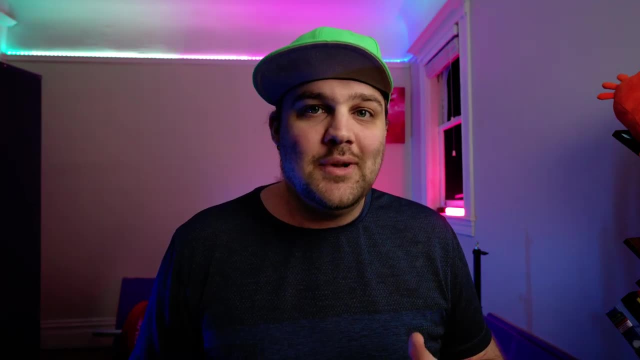 routing service functionality already exists and can be shared between Axum and other frameworks. So, with the data migrated in our last video and our web framework of choice chosen, it's time to actually build the API. The previous iteration of this API was built on top of AWS AppSync's. GraphQL support, but I decided to not go to GraphQL this time and, to be honest, it's not actually the fault of GraphQL. I actually really just want to remove AWS Amplify from my project and reduce the page weight that my users have to incur when they load the page. The core benefits of AWS's AppSync. 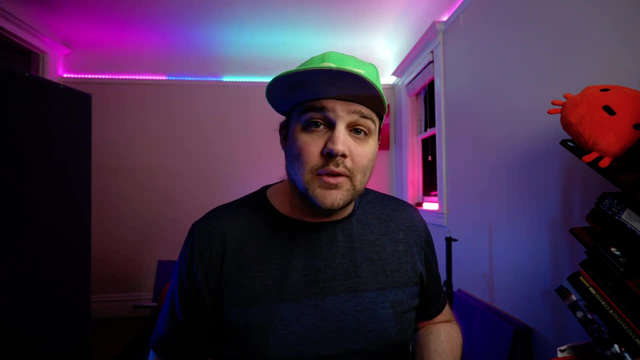 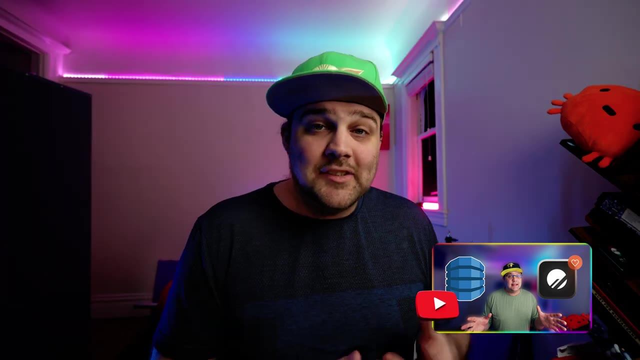 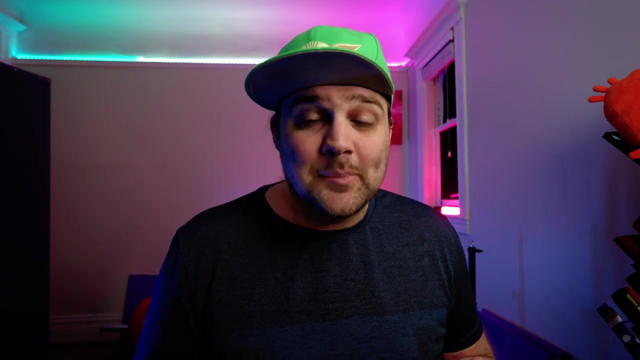 GraphQL implementation was deep integration, which means I have to figure out how to integrate with DynamoDB. But since I'm moving away from AWS anyway, I've already given that up with my choice to move to PlanetScale, Since PlanetScale, of course, doesn't have a deep integration with AWS AppSync. The other big reason that I liked AWS AppSync was 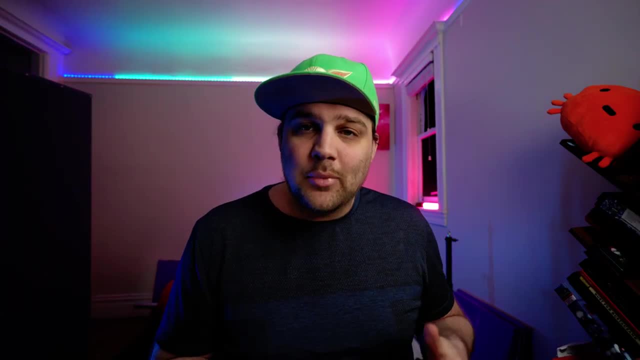 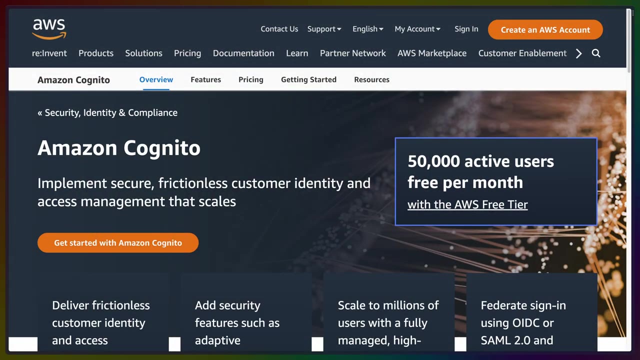 its deep integration with Cognito. But I'm going to have to solve that problem anyway, because I've chosen to move some things away from AWS already, which means I have to figure out how to interface with Cognito on my own. There are a bajillion examples and yes, that's a real number. 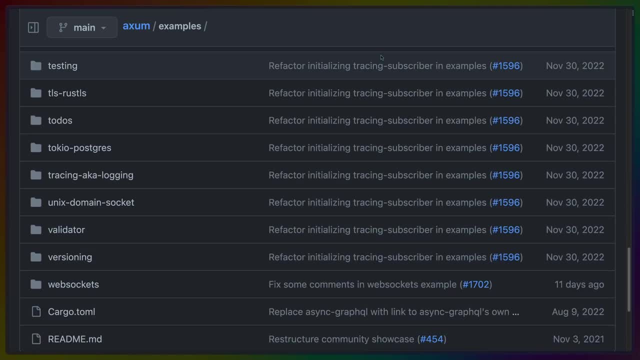 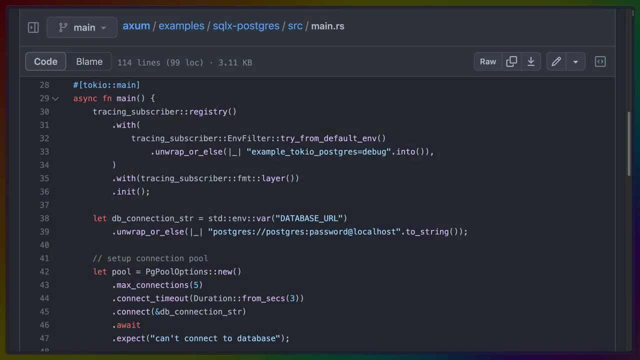 in the Axum GitHub repo, so it would be really hard for me to deny myself one of these. as a starting point for the code that I want to write, I chose to modify the SQLX Postgres example, as it's the closest to what I actually want in the end, which is SQLX and MySQL. This required 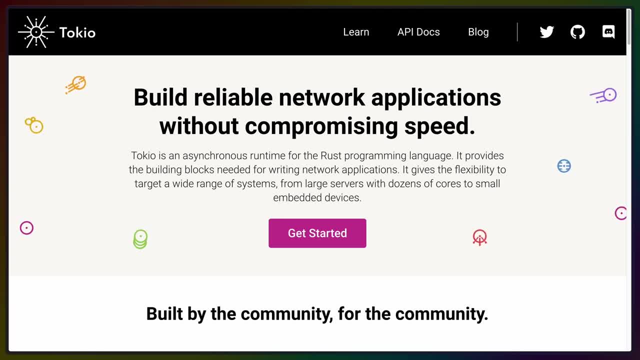 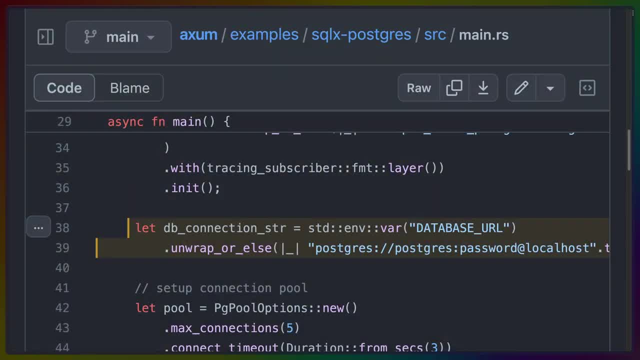 installing the Tokyo Tracing Crate, which is fine because that's what I'm going to use to monitor and observe my services anyway. There were some conventions in the example that I either didn't agree with or didn't need, such as needing to fall back to a local database if the remote database 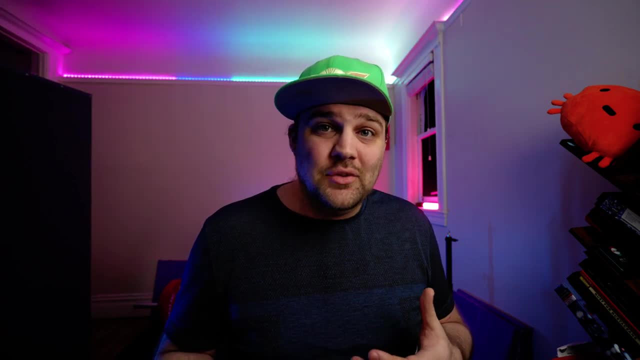 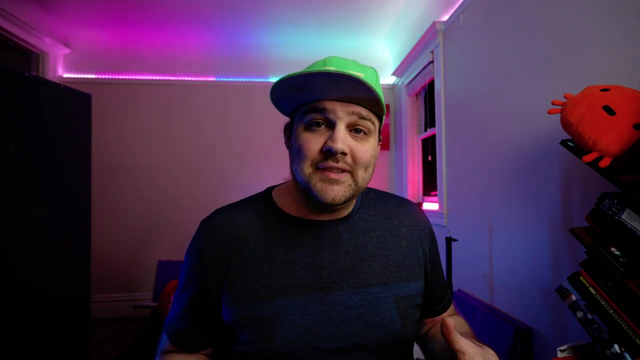 wasn't set. I don't really want my production application to try to access a local database if I forget to set the environment variable. I just want it to crash, so I removed that. There's also some fixes that will have to come later, such as replacing socket adder, which